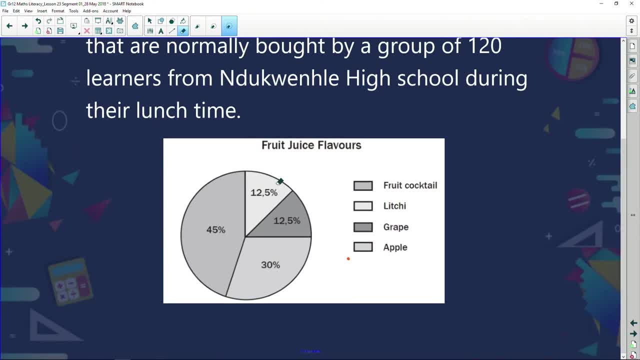 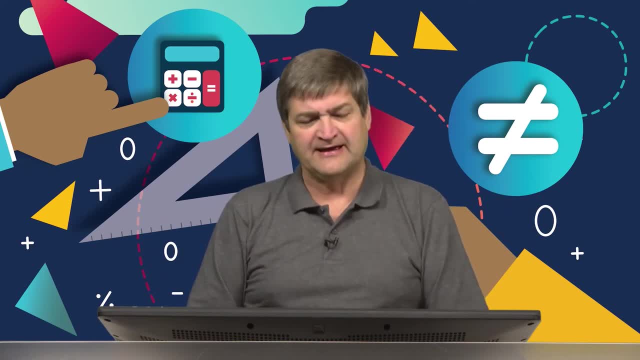 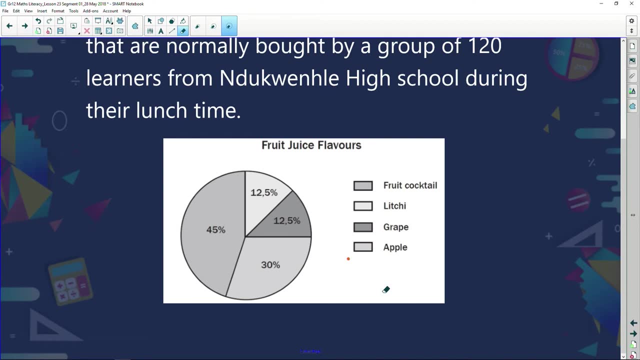 Notice our circular little graph. No longer bars, now circular. And the thing I love about a pie chart is straight away we can see how much one thing takes up of the whole. For example, we can see that this color, this light gray shade here, takes up quite a bit of the whole. So whatever. 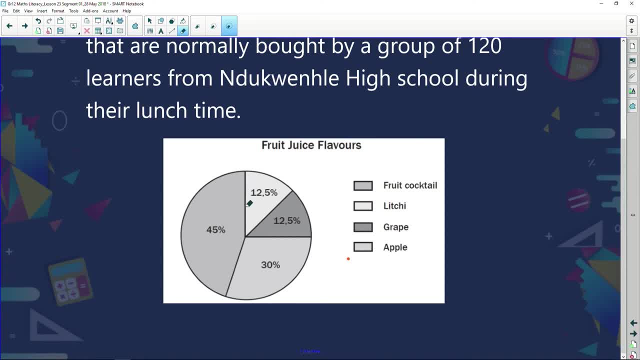 this is. it's really popular amongst kids. It takes up a big area. What is this? Well, now we have a key, and our key actually tells us that, if we look at this, this color here represents 45%, So 45%. 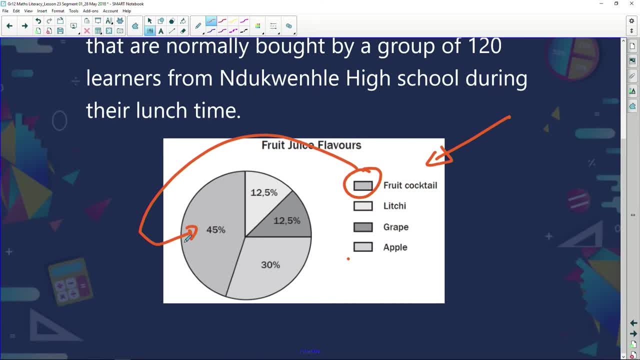 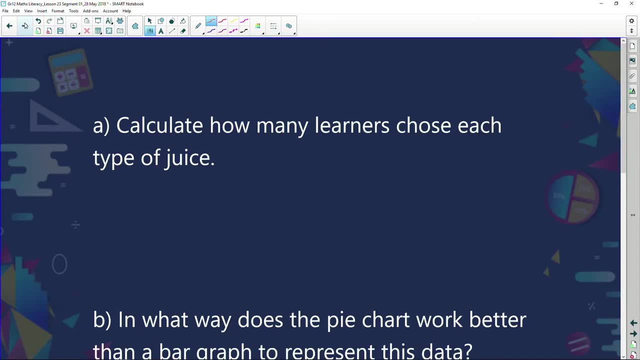 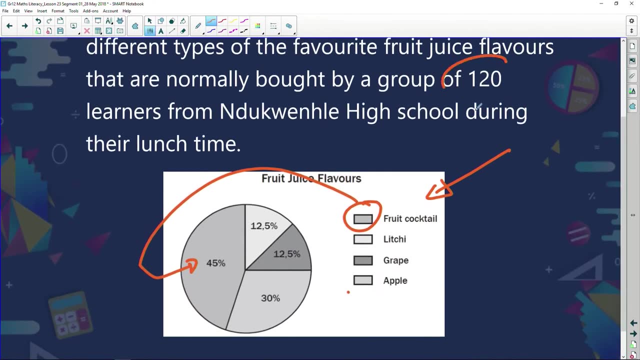 of our students love fruit cocktail juice. No longer bars now circular. So let's read questions. Calculate how many learners chose each type of juice. Let's have a look. How many learners do we have? We've got 120 learners. 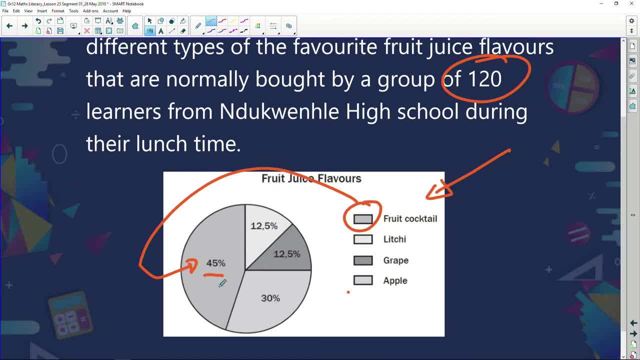 Of those 120, we know 45% love fruit cocktail, So 45% and guys, 45%, percent hundred, Okay, first thing that jumps to mind. So 45 over 100 multiplied by the 120.. So I'm going to say I've. 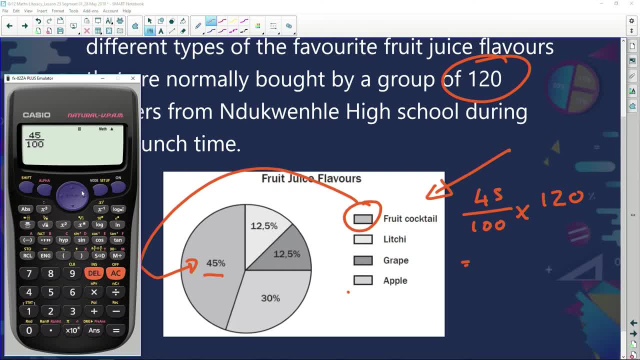 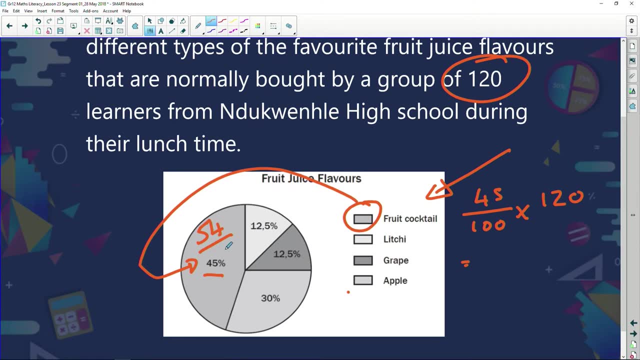 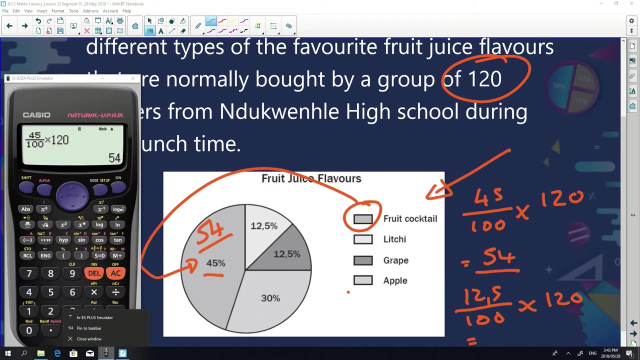 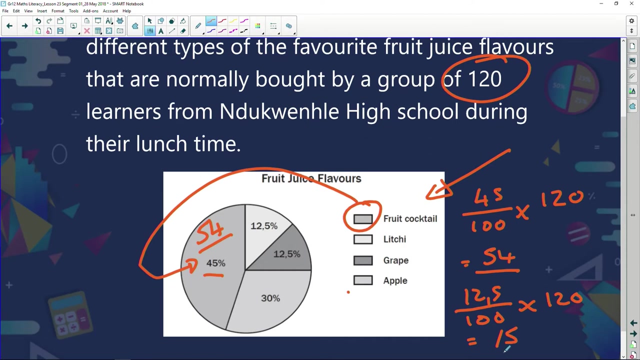 got 45%. Multiply that by my 120. And I get an answer of 54.. In other words, 54 students love fruit cocktail juice. Now let's work out: So 45 is 12 and a half percent. So 12 comma five over 100, because we're dealing in percent times 120.. Out comes the calculator and we say: right, Mr Calculator, 12.5 over 100, because we're dealing in percent. Multiply that by 120 learners and I'll end up with 15.. 15, what 15 learners? So 15 learners love fruit cocktail. 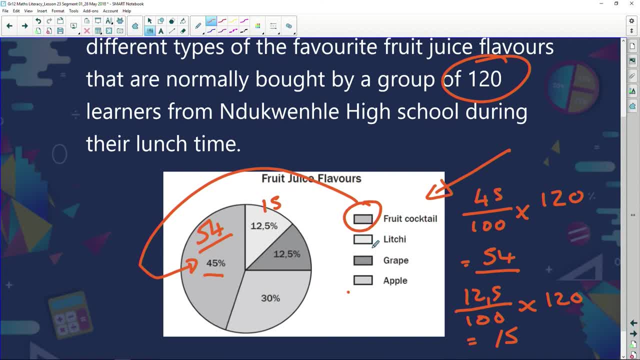 Does that work, True? 15 learners love sign language. Yeah, 15 learners love our lychee juice And 15 learners love grape juice. How do we know that? Because they're both 12 and a half percent. Now let's look at this: 30%. 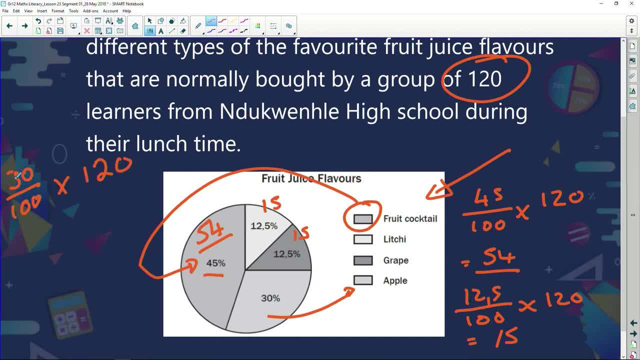 How many people like apple juice? Well, 30%. We got 30 over 100.. And again we're multiplying it by 120, because there's a total of 120 students. My calculator is going to do the work for me and it's going to say: right, we want 30% group. 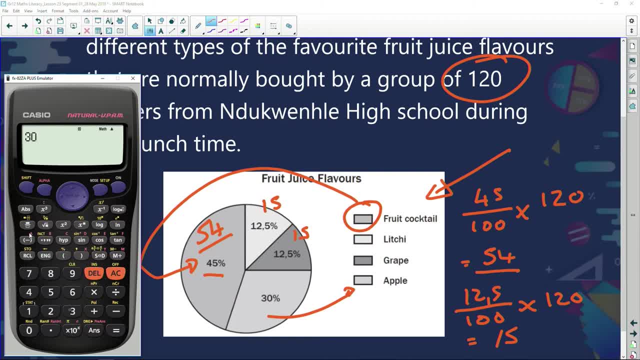 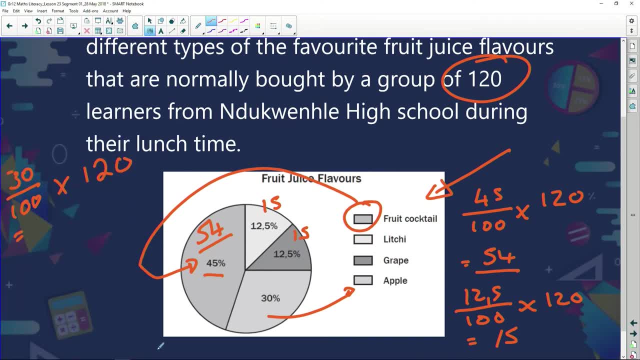 So 15 over hundred. There we go: 30 percent of 120 learners and i'll end up with 36. so there's 36 learners who love apple juice. now here's a way i can check whether my answers are correct, if i take these: 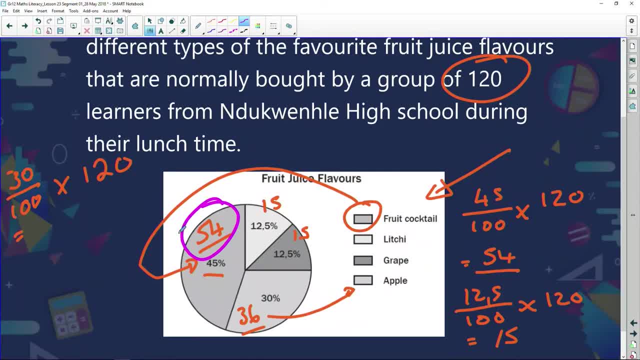 numbers of. let's just circle it here: 54 learners, 15 learners, 15 learners, 36 learners. it should add up to the 120 learners. if it doesn't, i've made a mistake, because you will see in this pie chart there's no little sector that's got nothing in. 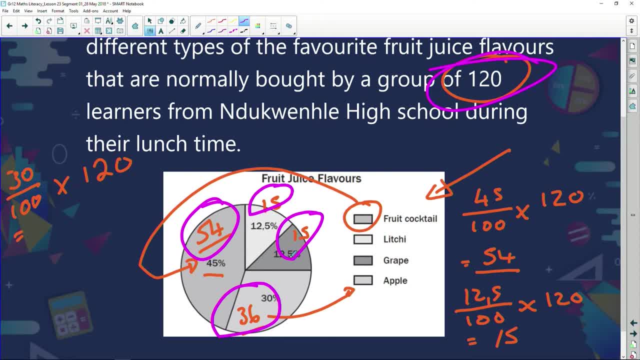 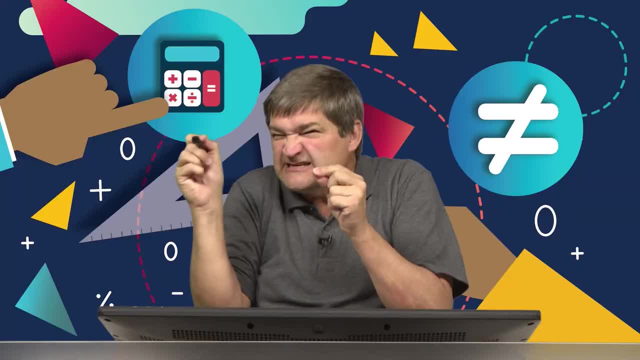 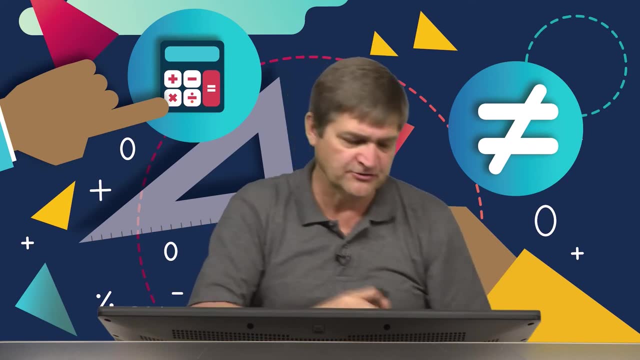 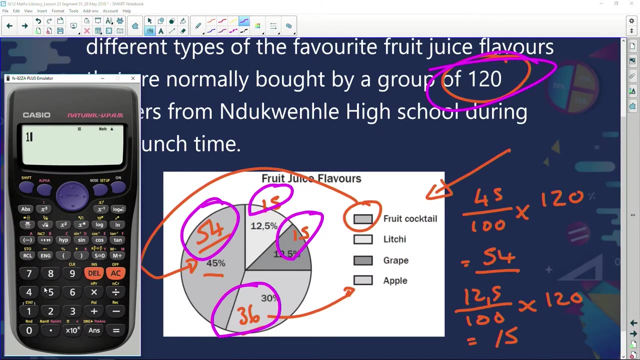 this pie chart is complete. it's complete with fruit cocktail, lychee juice, grape juice and apple juice. there's no little sector that says nothing. okay, everything. so all these sectors have to add to 120 learners. let's see if that is correct. so, adding up, we're gonna say i have 15. 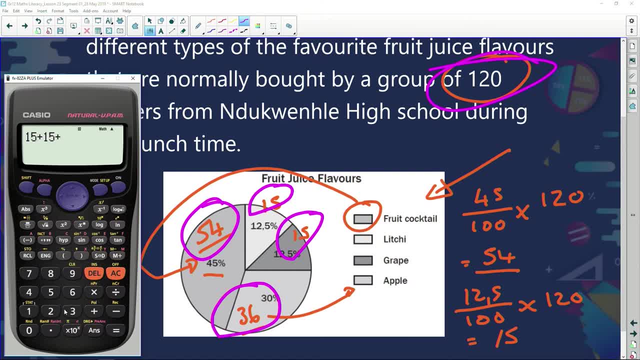 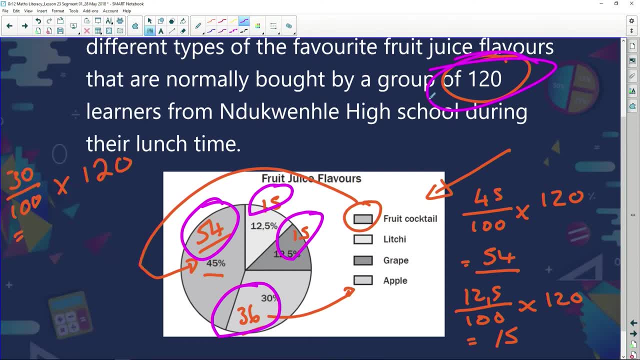 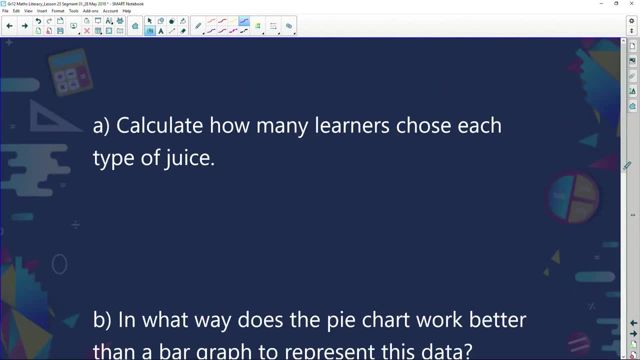 and i have another 15 learners, and then i have 36 learners and finally 54 learners. and voila, my answer is 120, which is a good thing, because i started with 120 learners. next question says: in what way does the pie chart work better? 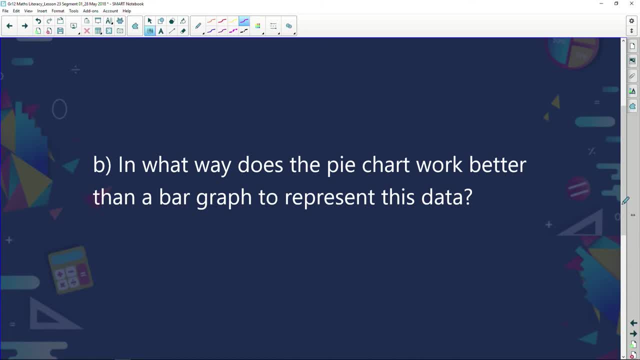 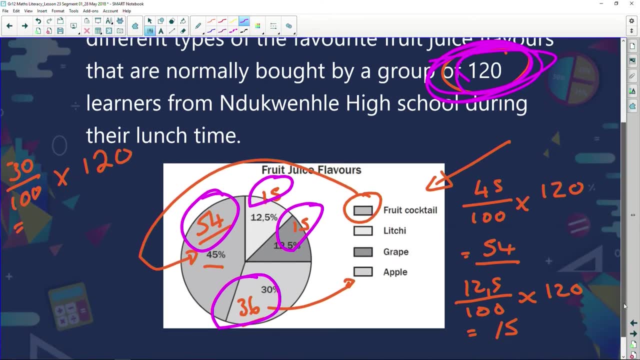 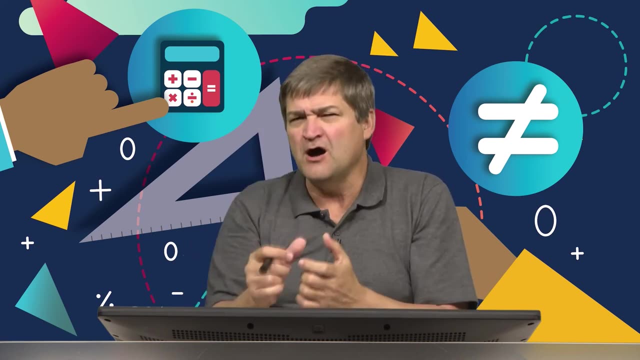 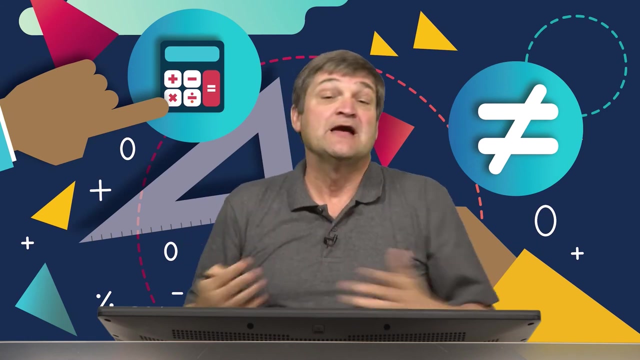 than a bar graph to represent the starter. so what is the advantage of a pie chart? well, a pie chart tells us exactly what percentage of learners like the juice, whereas if i had a bar graph, i would know the number of learners, but not the percentage of learners. and one of the advantages of having a bar graph is it gives me the 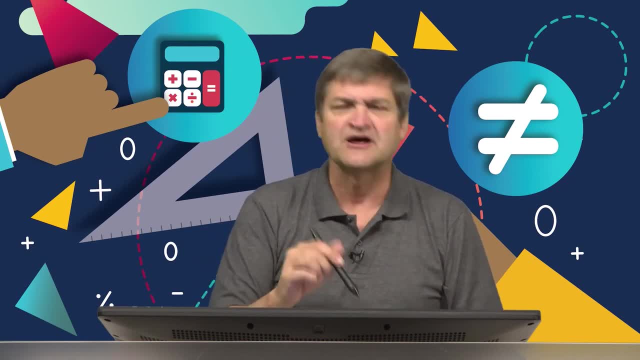 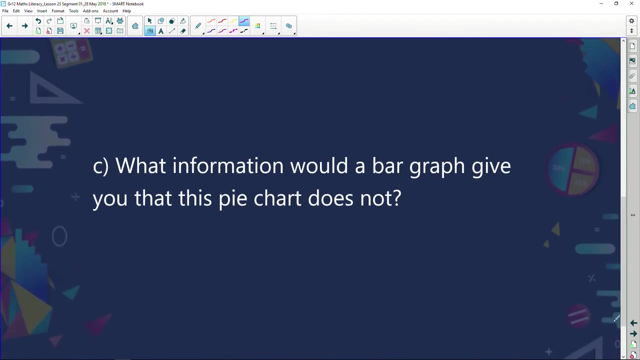 numbers where you can see in the pie chart. i had to work out those numbers. so all types of graphs have their advantages and have their disadvantages. okay, moving on. next question says this: what information would a bar graph give you then? this pie chart doesn't, and we've 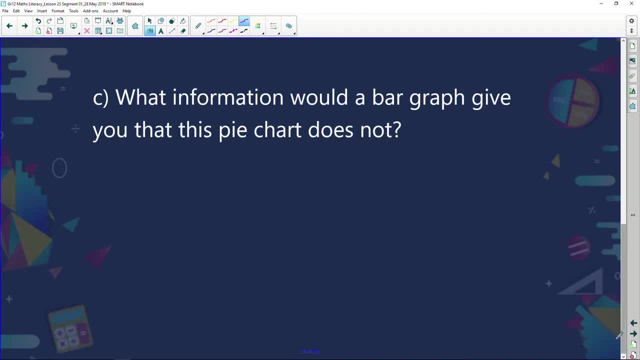 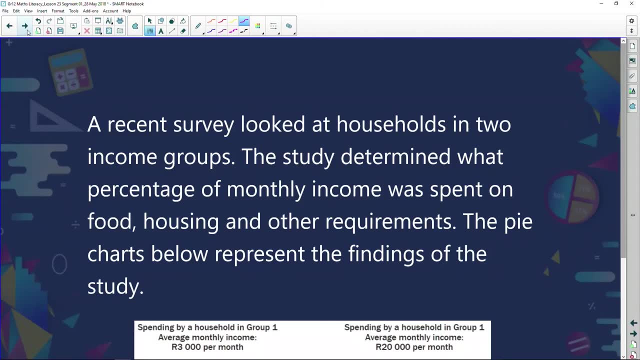 done that. we've said already it's to do with the percentages. here's another example, which is great. a recent survey looked at households in two income groups. the study determined what percentage of monthly income was spent on food, what was spent on housing and what was spent on other requirements. the pie charts below: 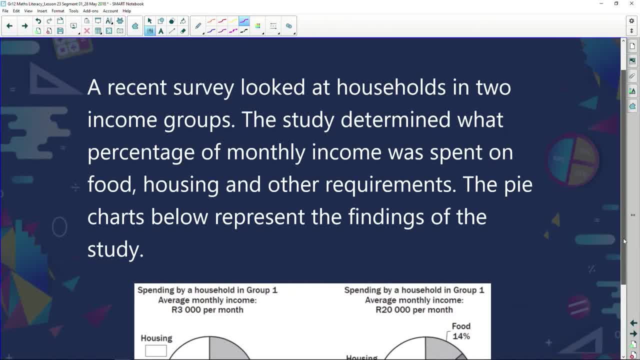 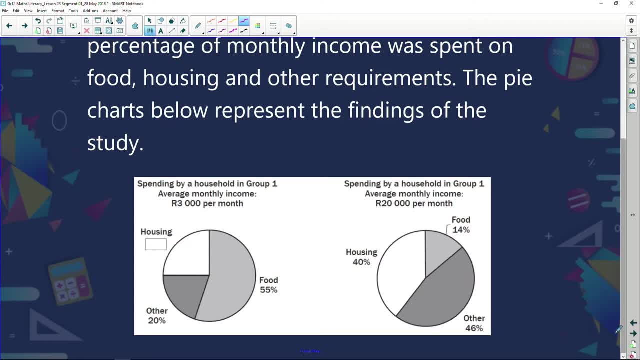 represent the findings of the study. so let's have a look here. we've got two pie charts. first one: spending by a household in group one, where their average monthly income is three thousand rand a month. next one, the spending of a household in this group, where the average monthly income 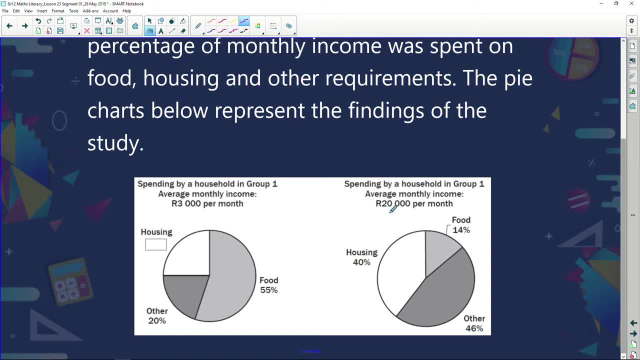 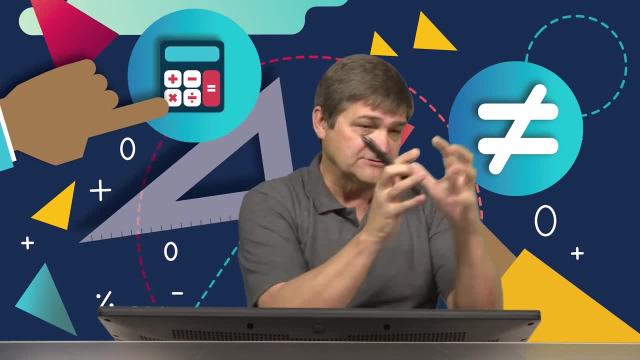 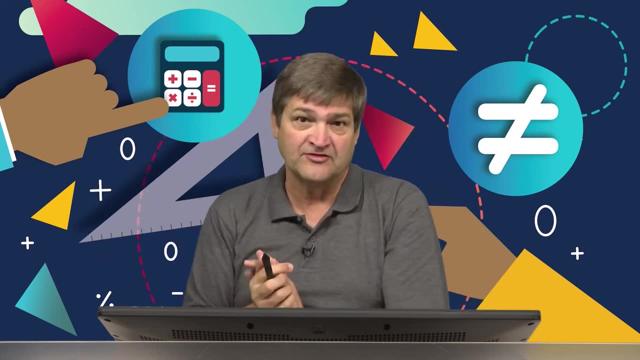 is now 20 000 rand per month. so we've taken a group of people and we said, right, let's take this group. we're going to look at those that average 3 000 rand a month and another group that averages 20 000 rand a month. 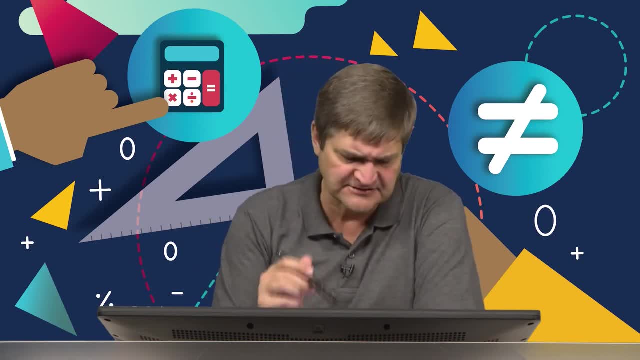 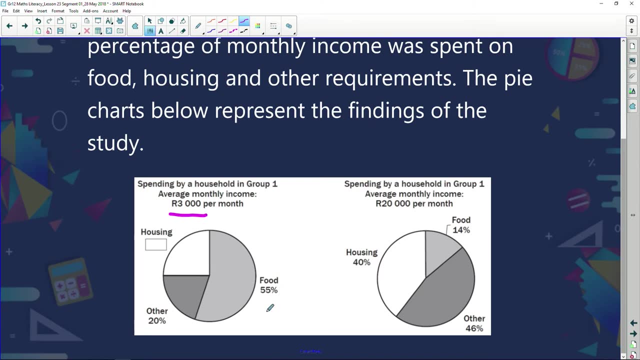 and see how they spend their money. so if you look at this, you can see that this household that earns an average of 3 000, they spend 55 of their salary goes to food, whereas these people that earn 20 000, only 14 of their salary goes to food- 20 percent here. 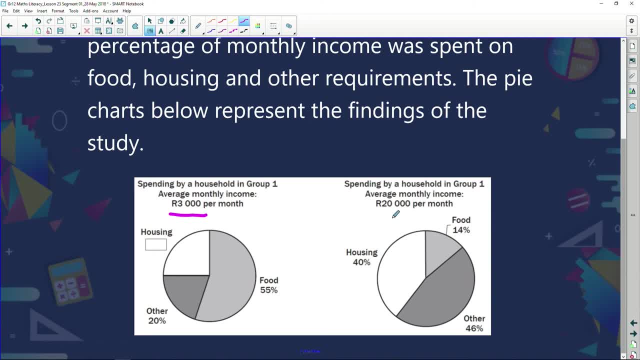 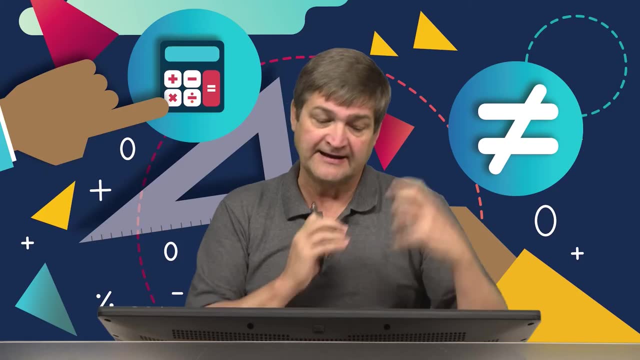 goes to other little things. when they earn 3 000, when they earn 20 000 other sort of requirements, they spend 46 of their money on those other little requirements. okay, now the two essentials are our food and our housing. okay, the other is all the other little bits and pieces. take note: the more 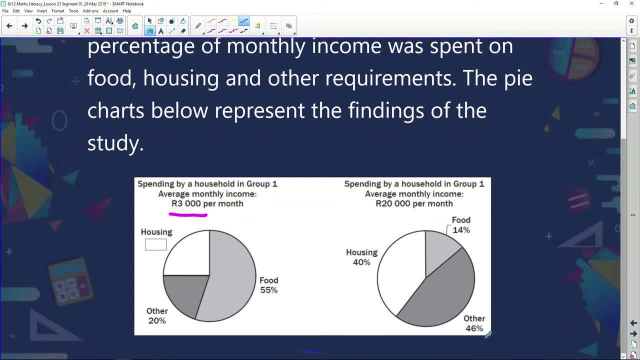 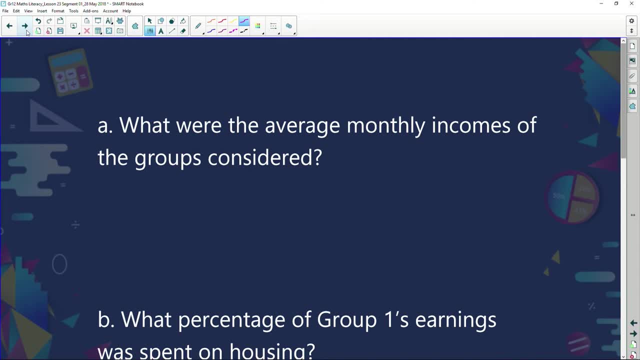 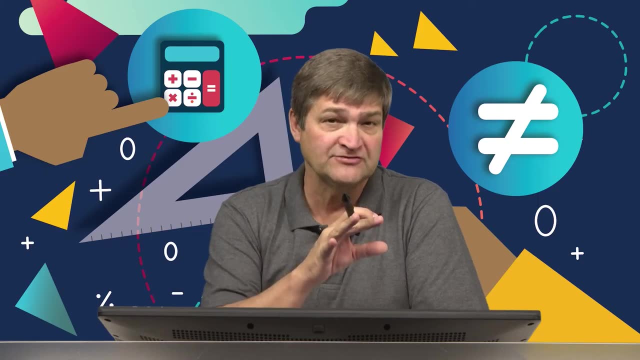 people earn, the more they spend on other things. right, let's work out, or let's have a look at, the type of questions and then try and work out the answers. what were the average monthly incomes of the groups considered? well, we've already said that one was 3 000 a month. 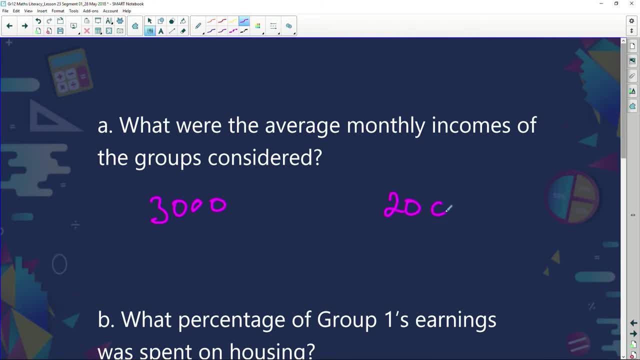 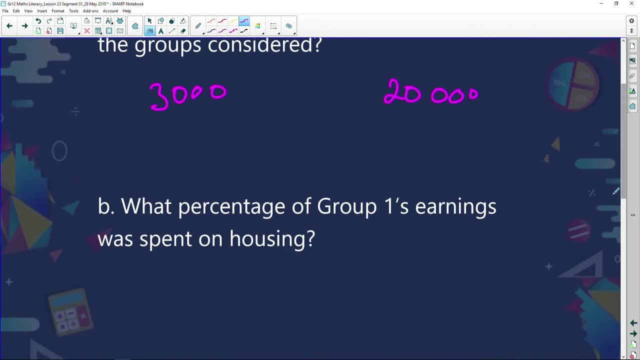 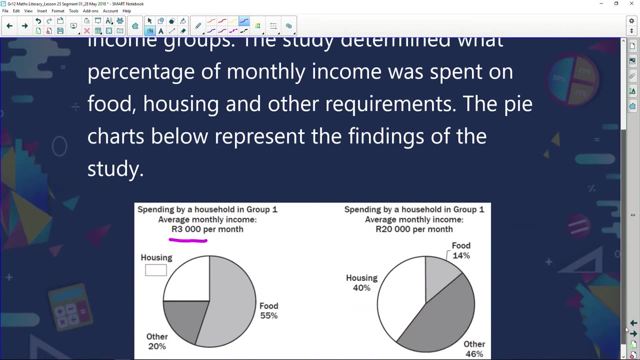 and the other was 20 000 rand a month. okay, what percentage of groups one's earning was spent on housing? okay, so let's go. group one: they said that they've got on housing. we've got to work it out now we know this is 55. 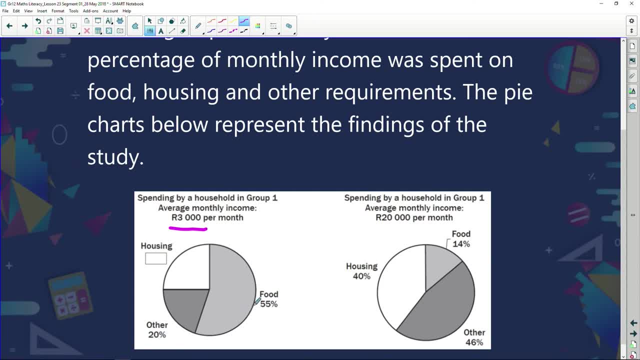 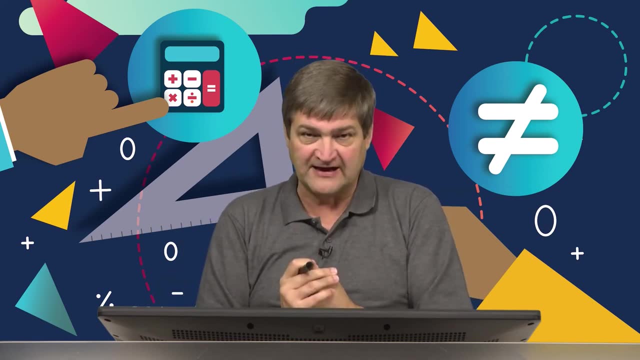 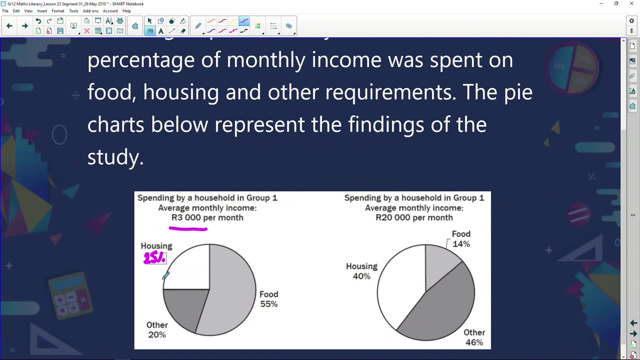 and this is 20, that makes 75. if that is 75, then this must be 25. why? because percentages add up to 100, and if i say 100 minus 55, minus 20, i'm going to be left with 25. so 25 percent of these. 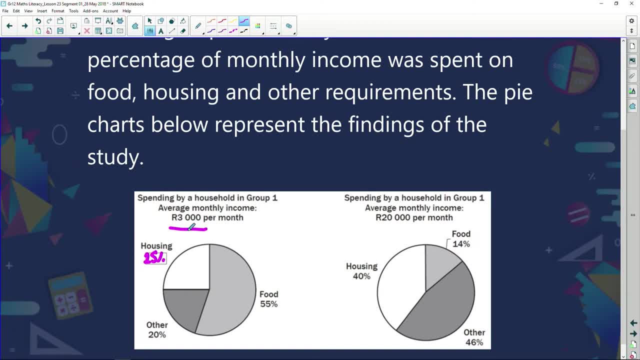 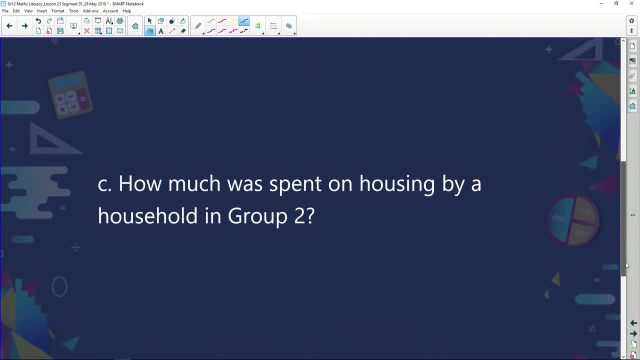 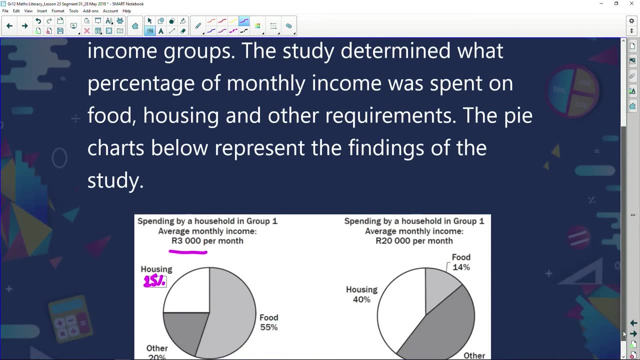 people's income is spent on housing. all right, that was nice and easy to do, wasn't it? next question: how much was spent on housing by a household in group two? so let's have a look here. here's our second group, and how much was spent on housing. it says: 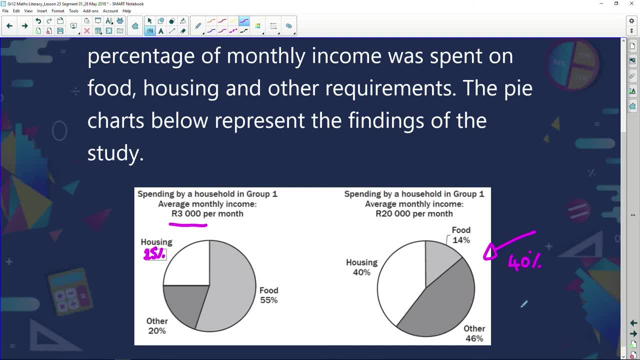 40 percent was spent on housing, and 40 percent of what? of the 20 000 rand a month. so we're going to say, right, 40 over 100, because we're dealing with percent multiplied by 20 000. let's have a look here quickly. 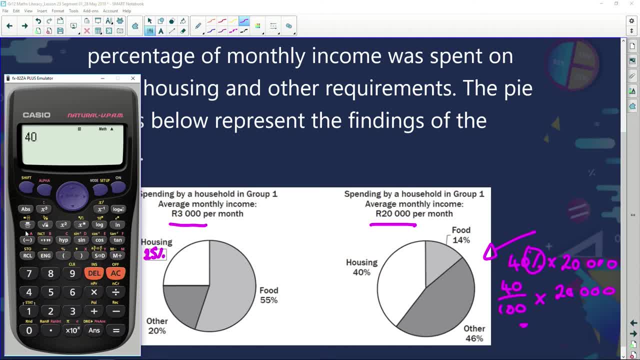 we're saying: right, sir, we've got 40 percent, so it's 40 over 100. then we're going to multiply that by 20 000 and we land up with an answer of 8 000. so they spend 8 000 rand a month. 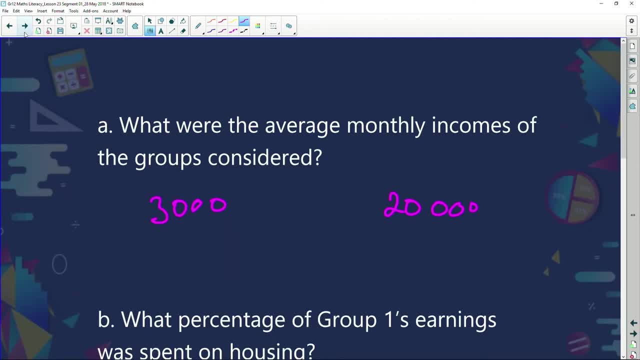 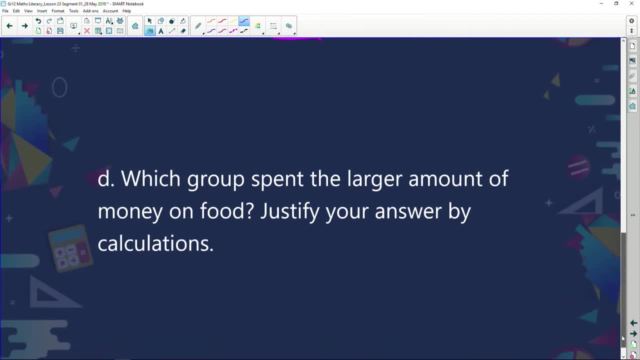 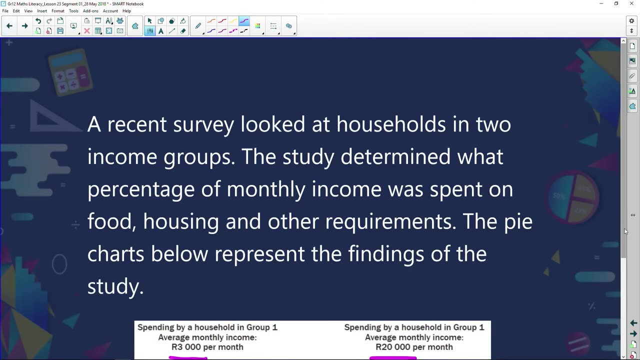 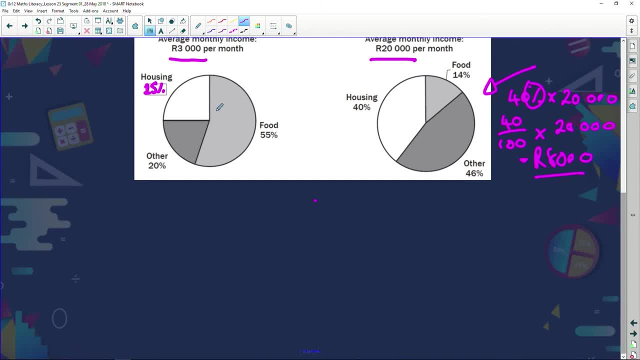 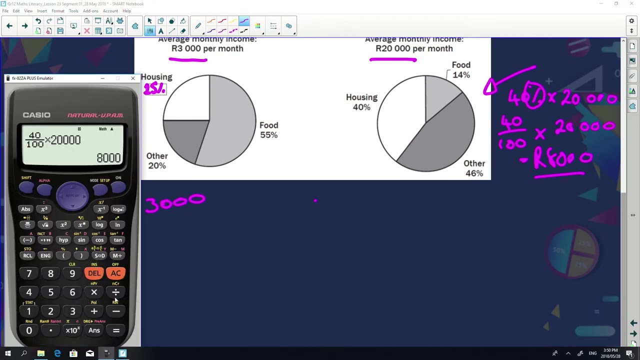 look at the food. we're going to look at this group, this group. they spend 55 percent on food, and 55 percent of what? 55 percent of this, of this salary of 3 000 rand. so we're going to say, mister calculator, we need your help, we want 55 percent. 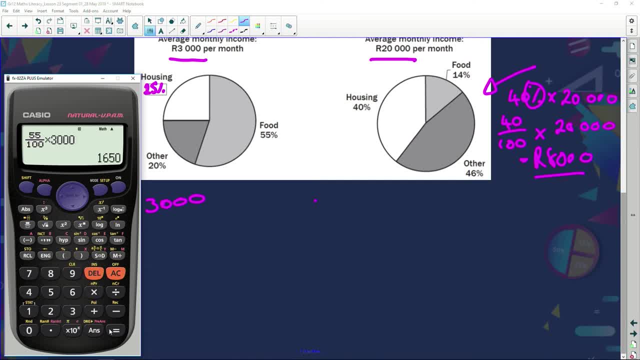 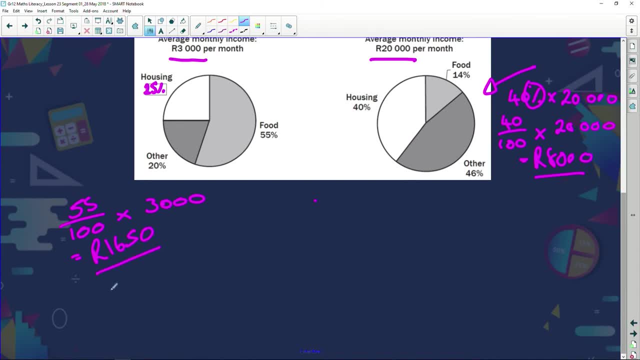 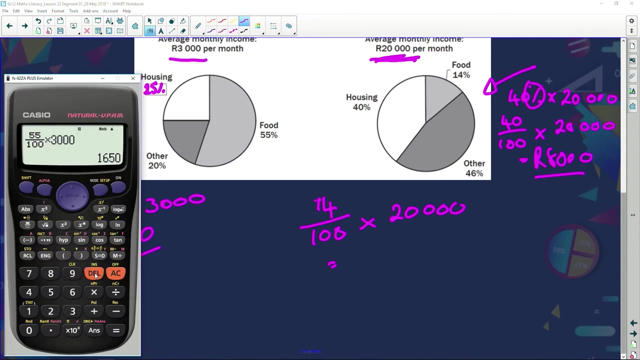 of 3 000 rands and we get an answer of 1 650 rand. okay, now this household only spends 14 percent of their salary on food, but they've got a bigger salary- 20,000. so now we're going to try and calculate 14%, or 14 over a hundred, and 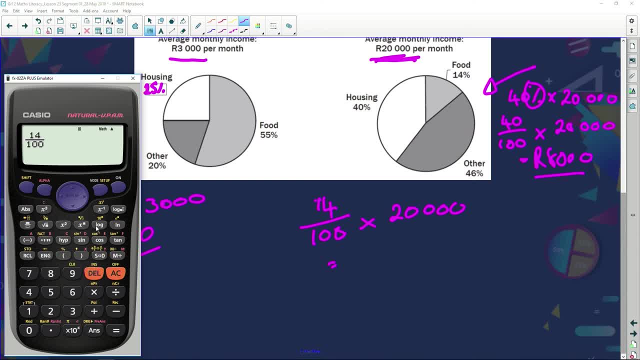 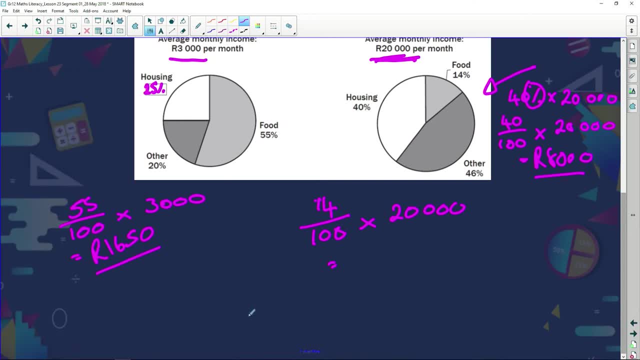 we're going to multiply that then- oops, let's just go back. we're going to multiply that then by 20,000, okay, and our answer is 2,800 red whoa, fuck. let's look at this. although this is a smaller percentage: 14%, and this is 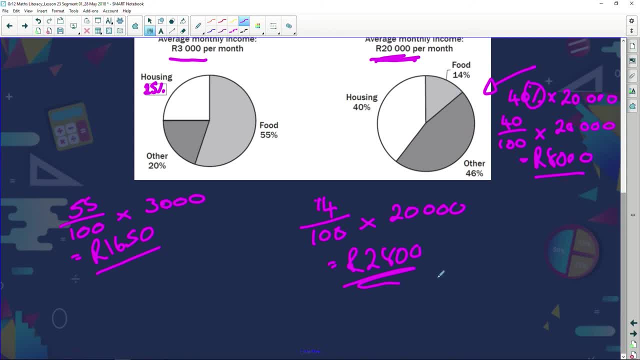 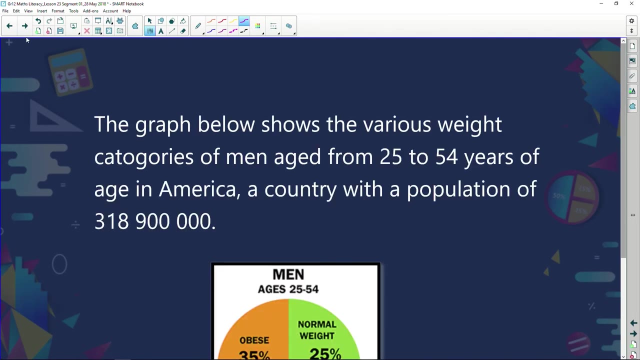 55%. the amount is a lot bigger, why? because at 14% is based on the 20,000, whereas this 55% is based only on 3,000 red. okay, interesting stuff, and we can just get this information from our graphs. let's have a look at this graph and we can just get this information from our graphs. let's 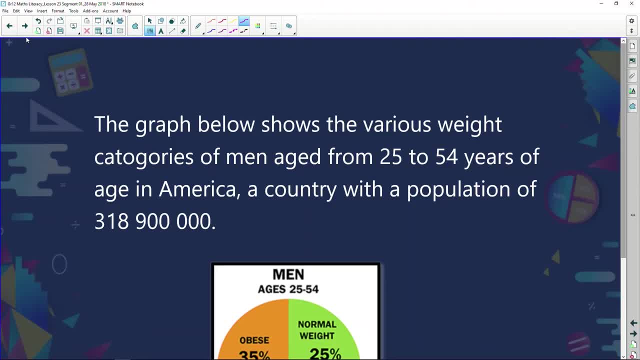 have a look at this graph, and we can just get this information from our graphs. let's have a look at this graph. the graph below shows the various weight categories of men aged from twenty five to fifty four years of age in America, a country with a population of 318 million nine hundred thousand. okay, so there is our bar graph. 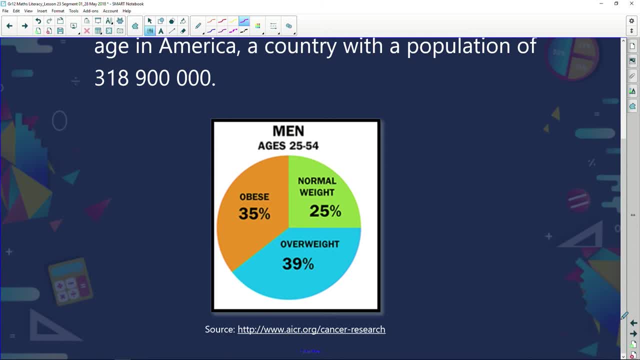 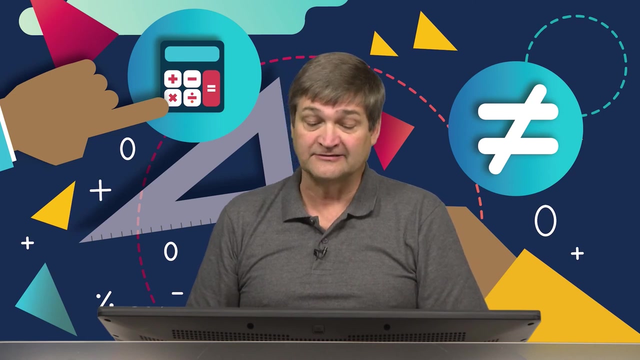 in it- sorry, our pie chart- and it shows quite clearly that 35% of men aged between 25 and 54 are obese and 25 are of normal weight and 39 are overweight. so it's quite a lot who are overweight and obese, whereas when you look at the normal weight, not that many, in fact. 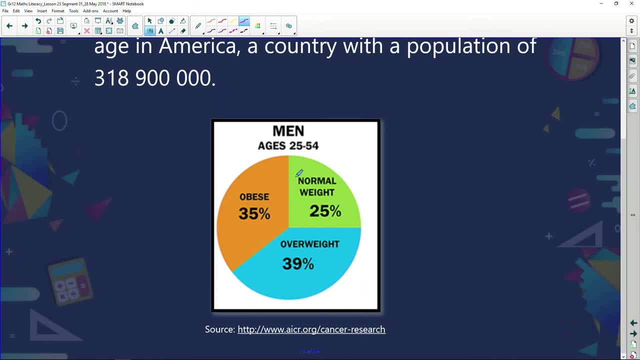 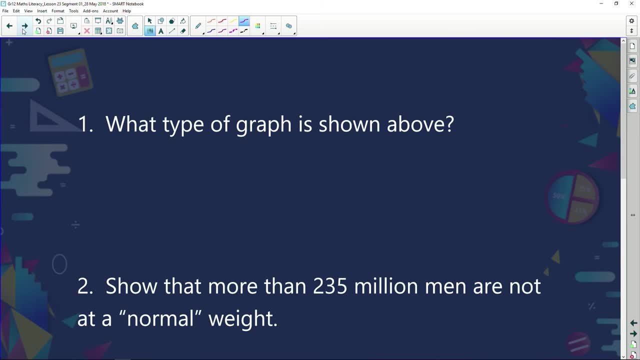 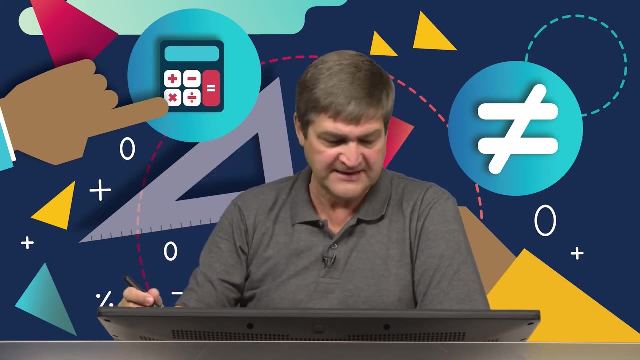 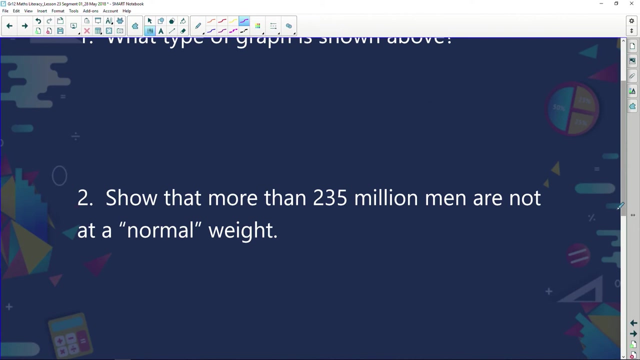 you can see, it just makes up a small segment or quarter of a segment, right? what sort of questions are they asking us? first of all, what type of graph is shown, guy pie chart. you know that it looks like a pie, it's round. next one show that more than 235 million men are not at a normal weight. now how many? 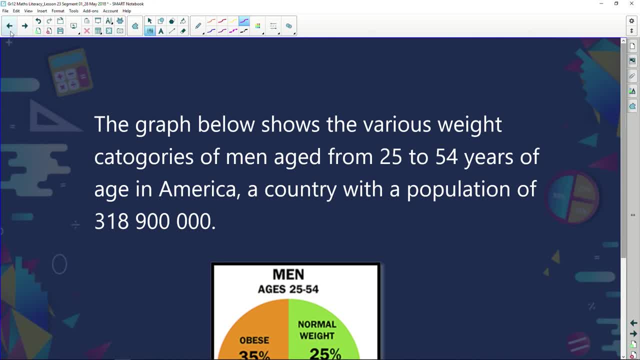 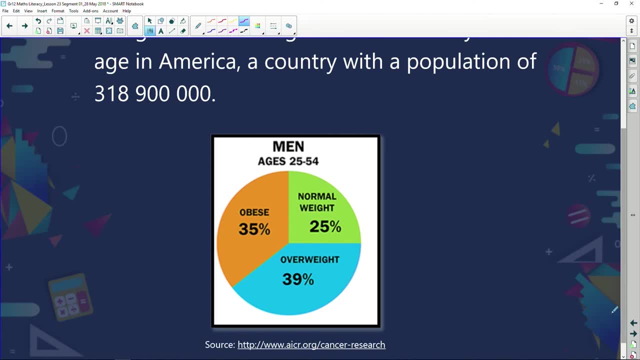 were not at a normal weight. let's go and have a look. normal weight is 25, which means there should be 75% percent left over. now I want to bring something to your attention. do you agree that this should all add up to a hundred percent? because percentages add to a hundred? now I'm going to show you. 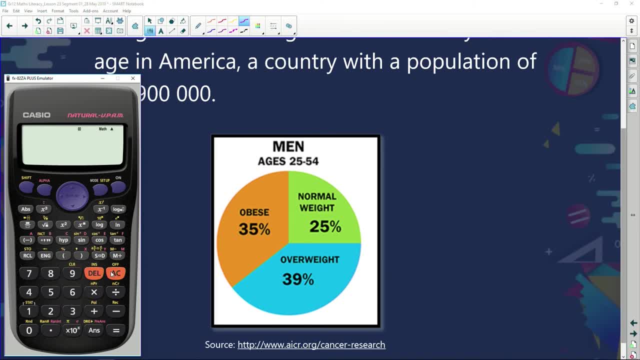 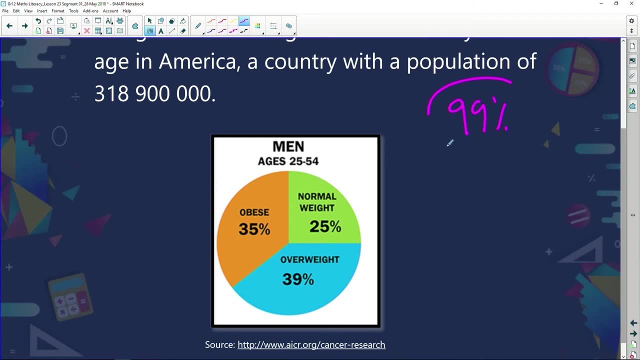 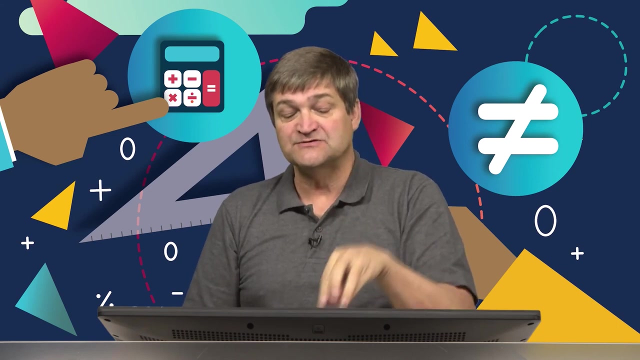 something interesting, and it's not a question, but it could well be a question in a final exam: 35 percent plus 25 percent plus 39 percent, and it gives you 99 percent, not a hundred percent. why, people? I'll tell you, because these percentages are obviously rounded. they probably rounded down a. 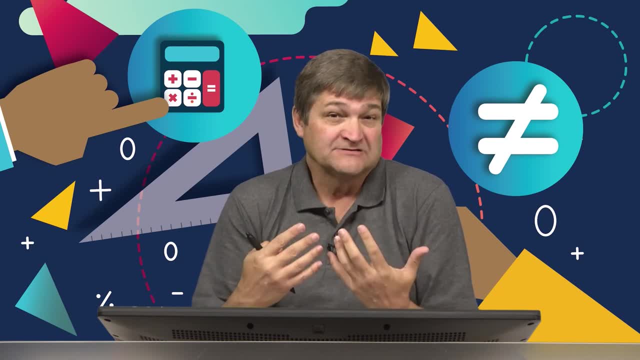 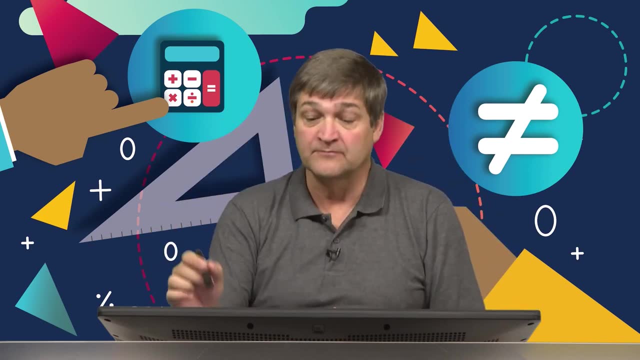 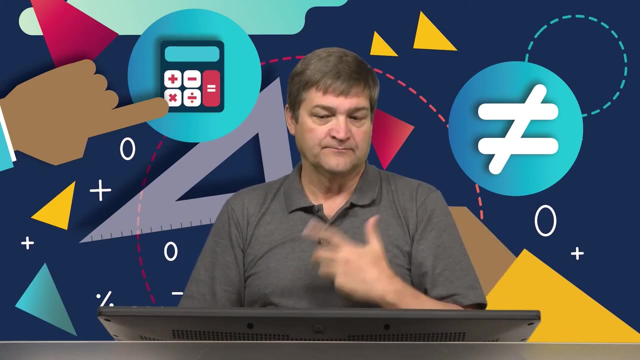 bit or round it up a bit. okay, some are rounded down, some round it up. in this case they've probably all or most of them have been rounded down, because we've landed up with a 99 percent and not a hundred. transcribers were at a high percentage for the rapid развитé og statistik reasons for this demographic破검idença. 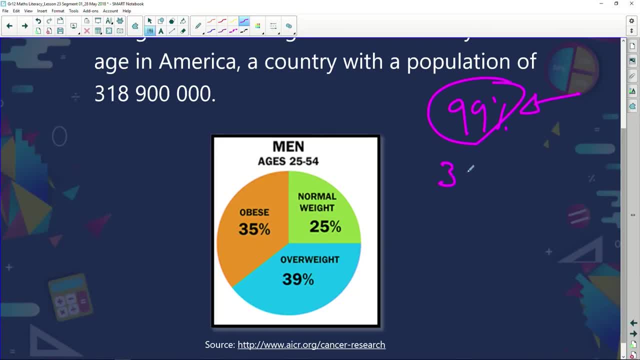 am, or most of them, have been rounded down because we've landed up with a 99% and not a hundred percent as well negative. we'd hope so. the 35 could have been, uh, 35 comma 4. it could have been 25 comma 4 and it could have. 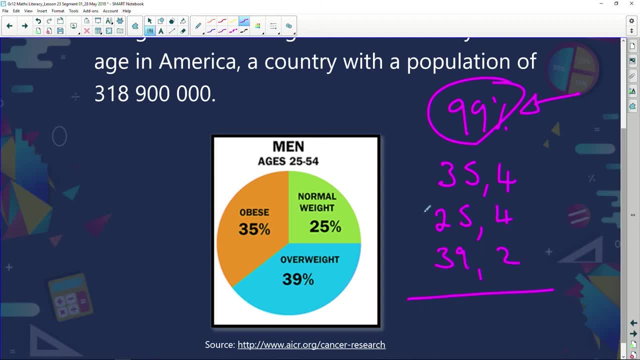 been 39 comma 2.. when you add those up now you're going to get a hundred percent. but you will see, these figures are whole numbers. in other words they said, hey, 35 comma 4, that's 35 rounded. 25 comma 4 is 25 rounded. 39 comma 2, that's 39 rounded, and this 442 would have made another. 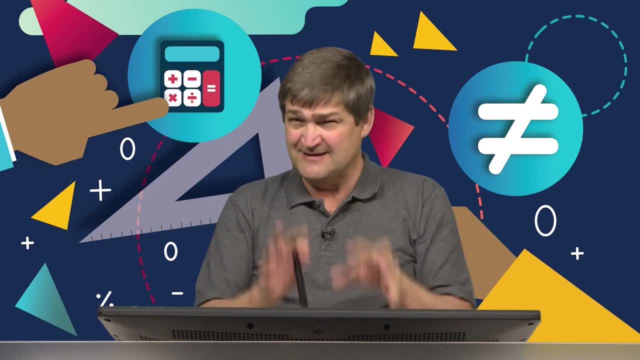 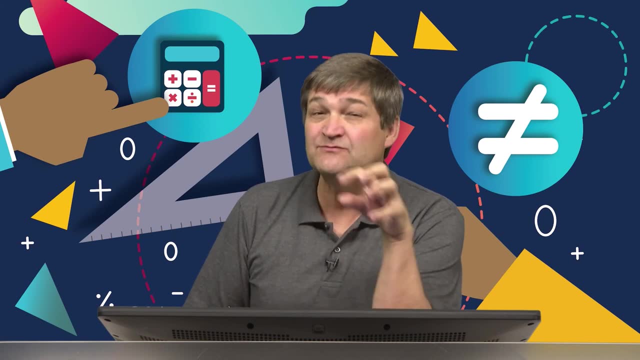 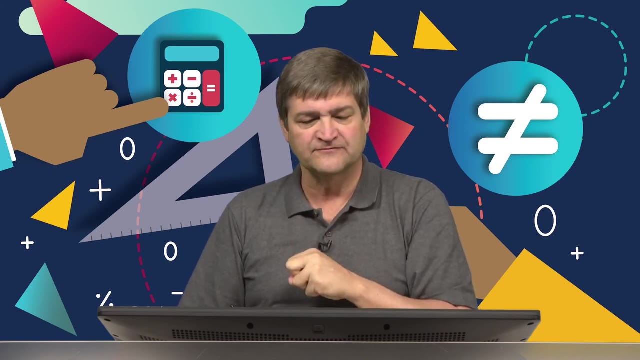 percent, which would have taken it to 99.. that's a deep question, hey, full of understanding that, but it can come up in exam paper. in fact, i've seen similar questions where it will say: how come this doesn't add to that because there's been rounding involved. okay, now our question is this: how many? 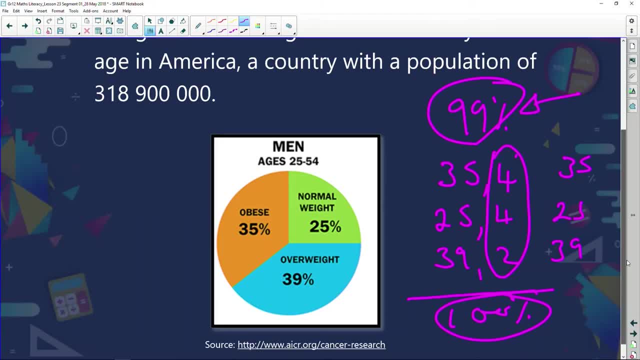 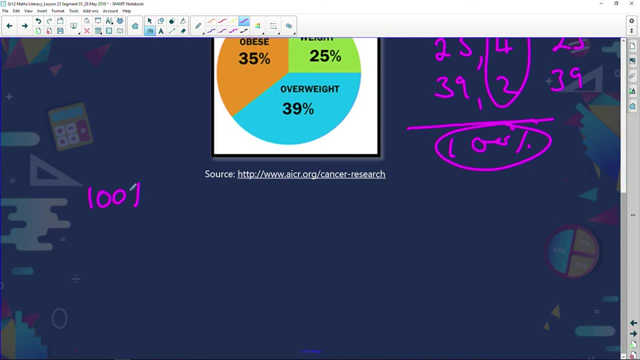 are not of normal weight. well now this your examiner would have to accept two answers. one you could say: well, a hundred percent makes up a power. minus the 25 percent means there's 75 percent that are not of normal weight. or if you'd added those two up, you could have got 35 percent plus the 39. 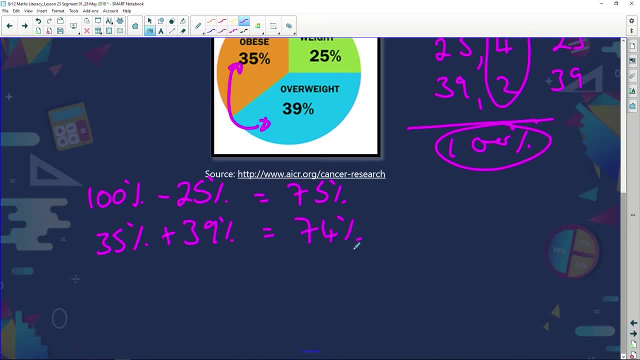 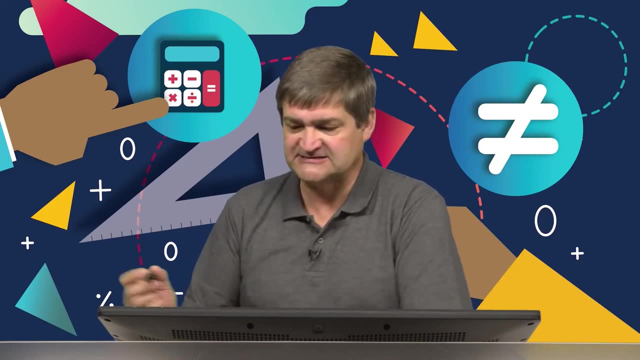 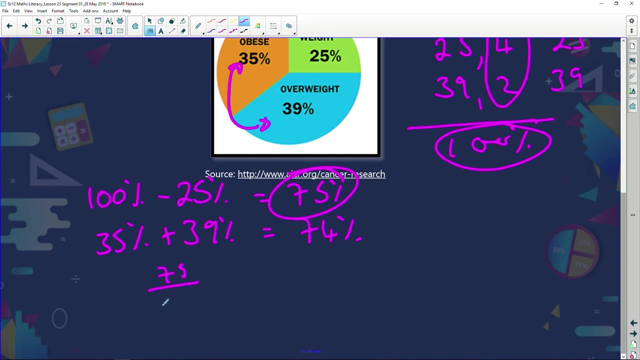 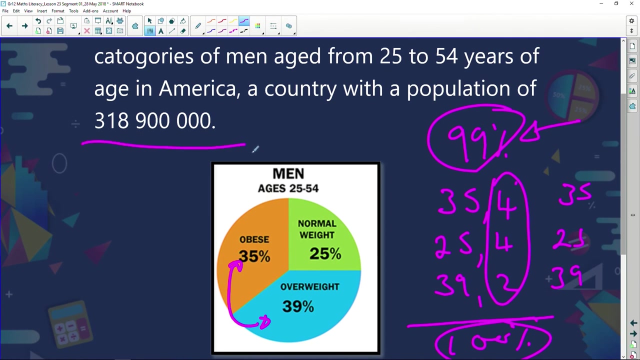 percent and you would have got 70, four percent. so the examiners would have to accept both answers here. all right, because it still shows understanding, but now let's work with the 75 percent. why? just because i want to. so 75 percent is 75 over 100 multiplied by how many men. we're gonna say 300, and they have said population and 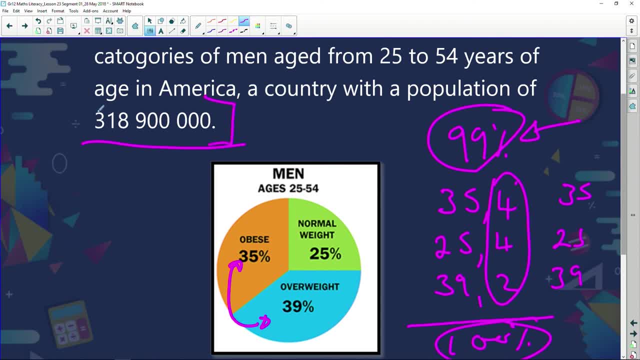 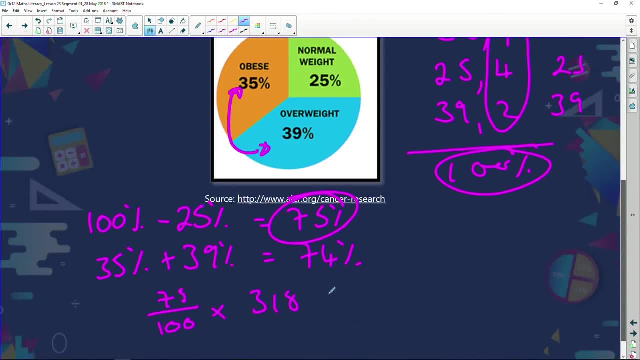 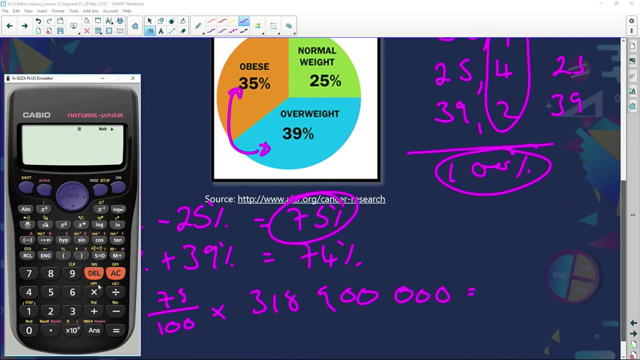 remember. we are looking just as men, so the question is a little bit flawed. but 318 million nine hundred thousand three hundred and eighteen million nine hundred thousand. okay, we multiply that. let's see what our calculator gives us for this: 75 percent, 100 multiplied by. 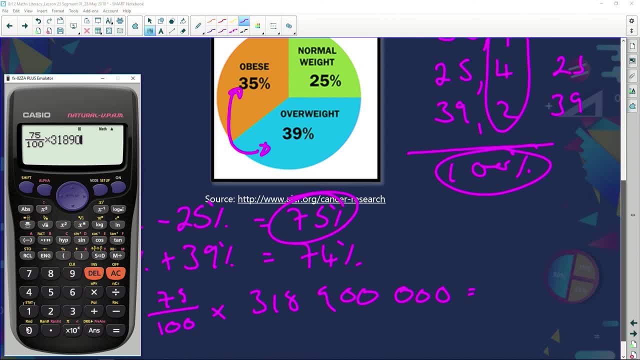 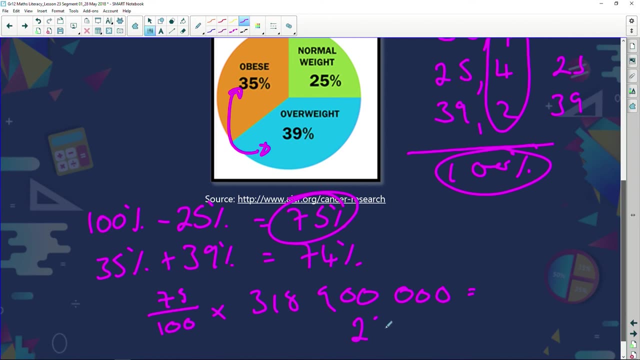 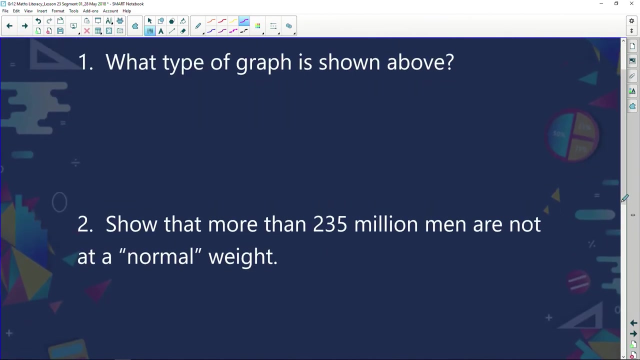 318 000, sorry, 318 million. 900 000 equals wallah, huge number: 239 million. a hundred and seventy five thousand. let's write that down: 239 million. and then it was a hundred and seventy five thousand. one, seven, five, zero, zero, zero. the question said: show that more than 235 million people, men, are not at. 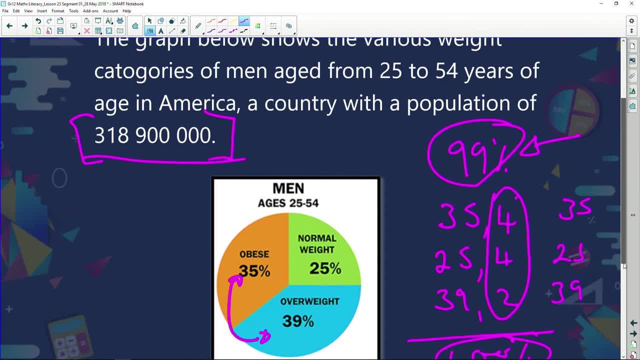 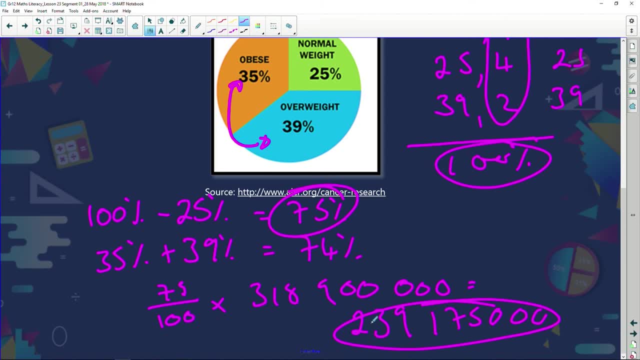 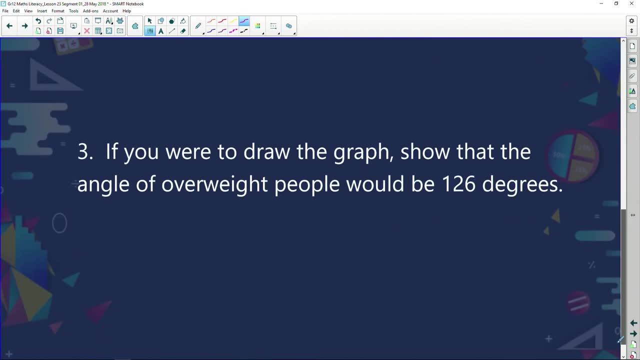 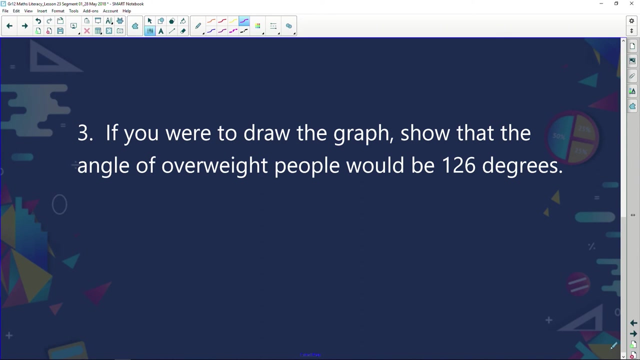 normal weight. so it's got to be more than 235 million. are we more than 235 million? indeed, we are okay. case closed, everything is proved right. then we look at another question. if you were to draw the graph, show that the angle of overweight people would be a hundred and twenty six degrees. lovely question this. 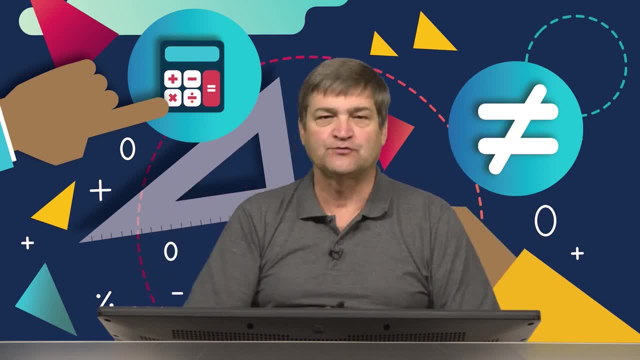 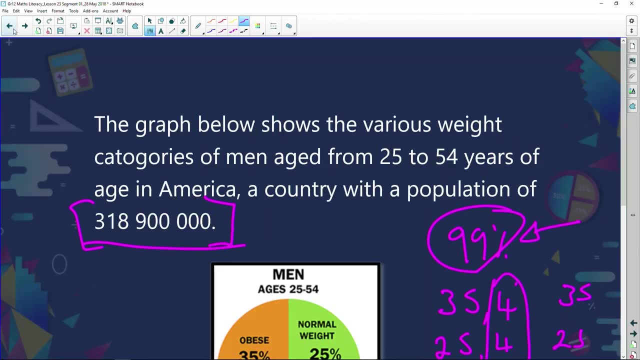 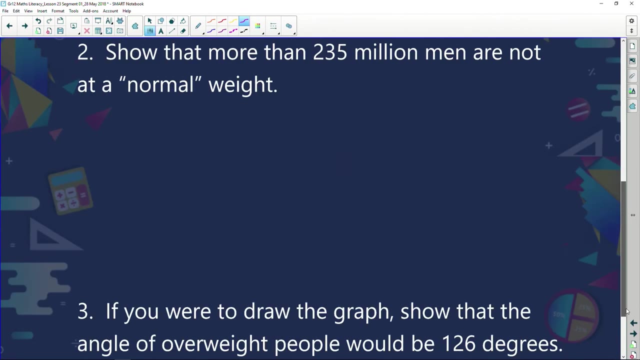 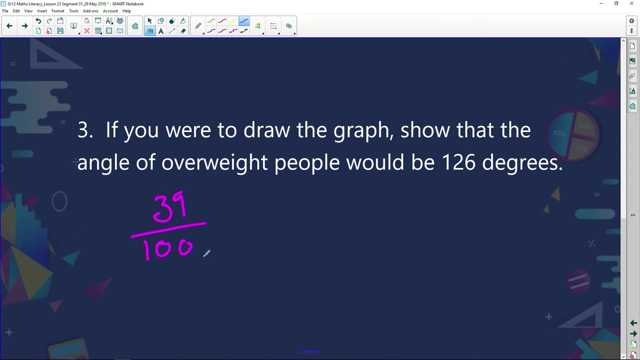 folk and even though we're running short of time, I've just got to do it with you because it's so important. okay, so how many people are overweight? if we go back, we can see that overweight people is 39%. so let's say, alright, so I've got 39%, and 39% is 39 over 100. I want to know how. 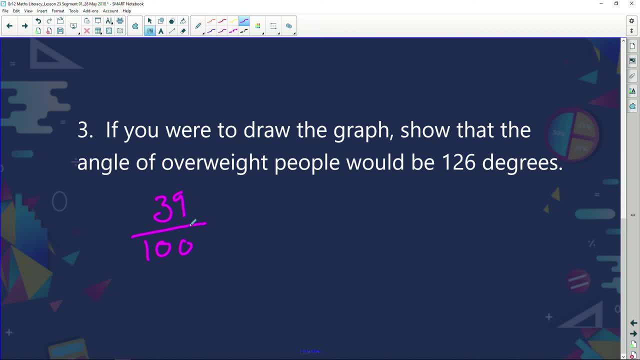 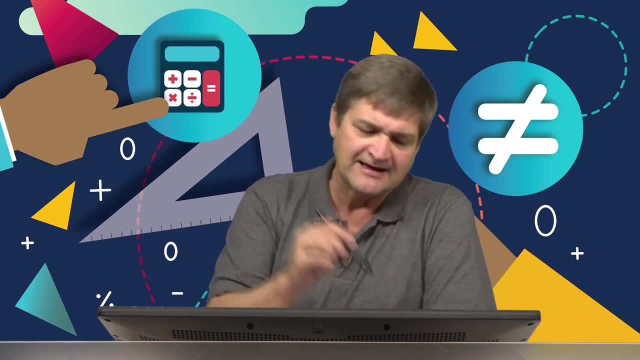 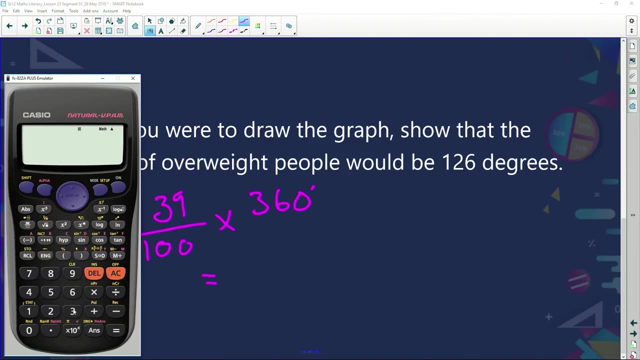 many degrees is it so? 39% of 360 degrees and folk, there are 360 degrees in the circle. so I'm trying to find thirty nine percent of that 360. so let's do it: thirty nine percent, thirty nine of a hundred, okay, multiplied by 360 degrees equals, and we get an answer of a hundred and forty. 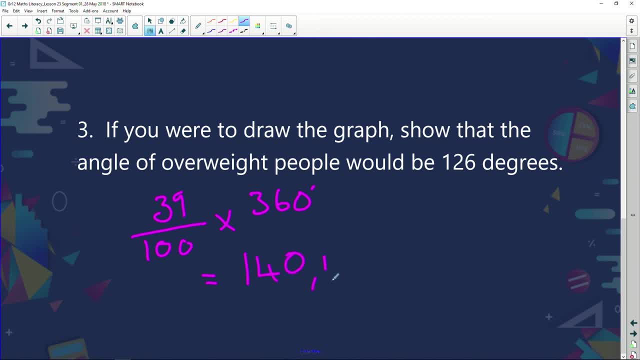 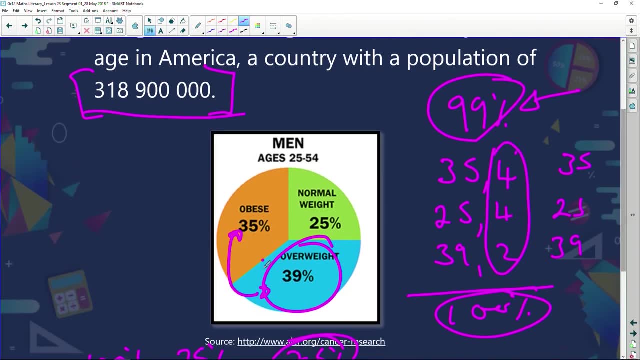 comma four degrees. a hundred and forty comma four degrees. so fuck, if I was drawing this this angle, yeah, I'd make a hundred, and let's use a different color so we can see it even clearer. I would make this a hundred and forty comma four degrees when, if I had to draw it- okay, normally for pie charts we don't.